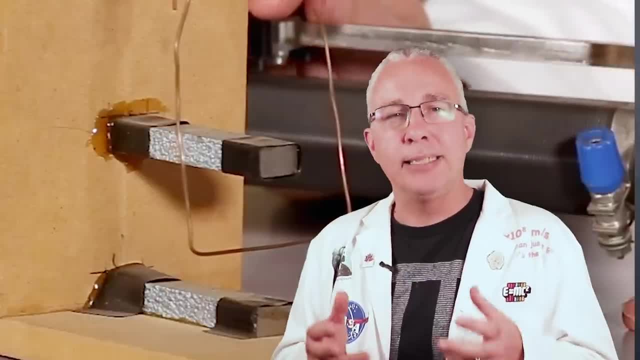 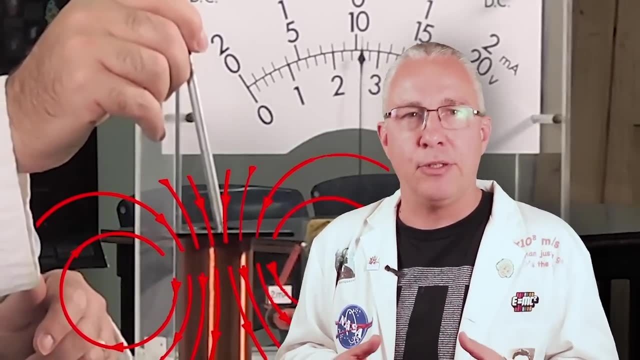 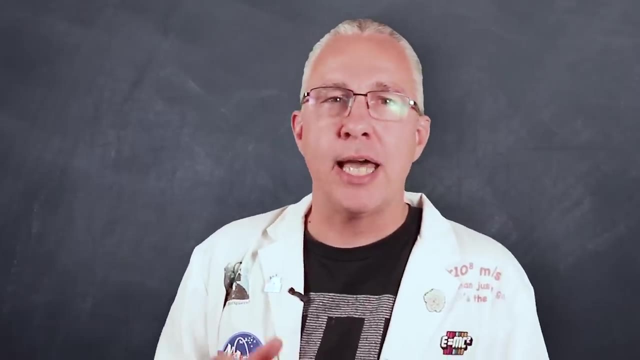 So he found out that a current bearing wire placed in a magnetic field will experience a force, And he discovered that when a wire experiences a changing magnetic field, or more correctly, a changing flux, it generates an EMF. But what Michael Faraday lacked was 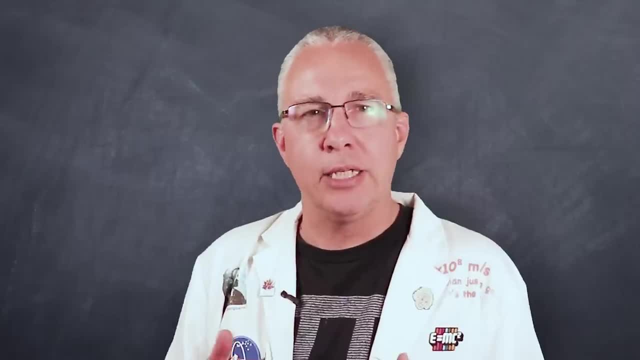 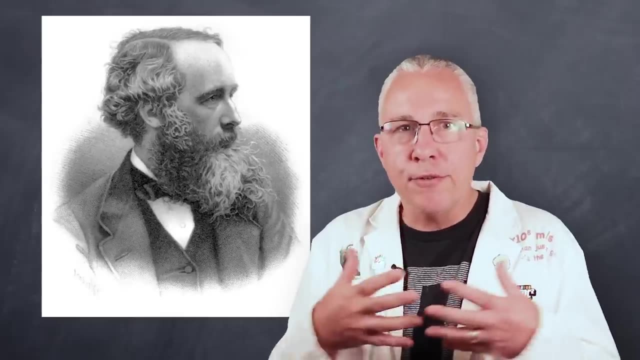 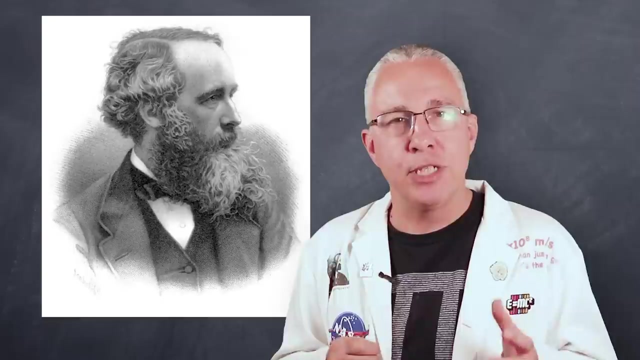 a strong mathematical foundation or background to explain the linkage between magnetism and electricity. So enter James Clerk Maxwell. Maxwell set out to unify these two separate mathematically, and he did so by examining four key equations that govern electricity and magnetism, and these became Maxwell's equations, And this is: 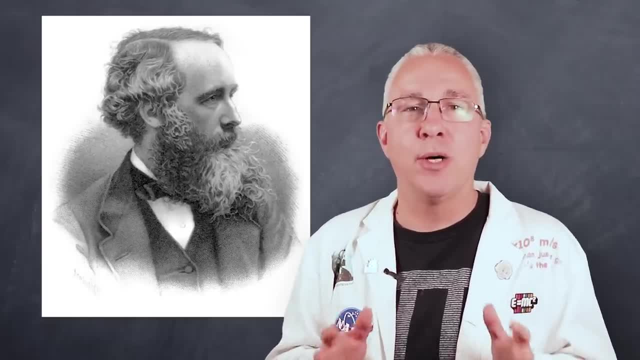 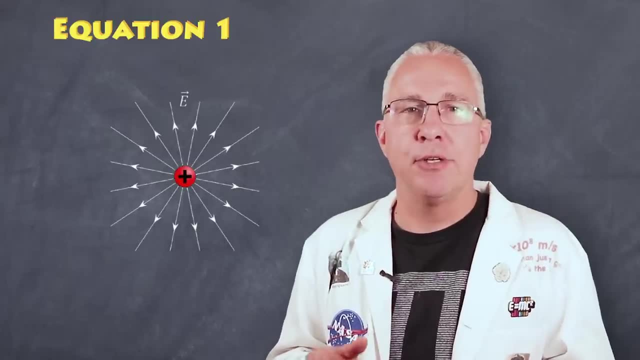 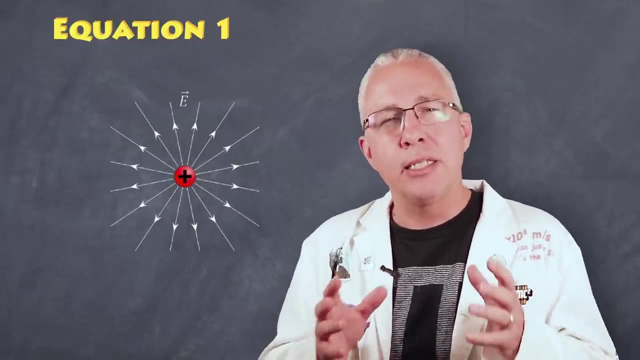 where the mathematics starts, so I don't want to stress you out. don't worry too much about the formulas themselves. The focus is in what they represent. The first equation is commonly referred to as Gauss's law and in essence it's describing the electric field around a point charge. Now in its simplest form, a. 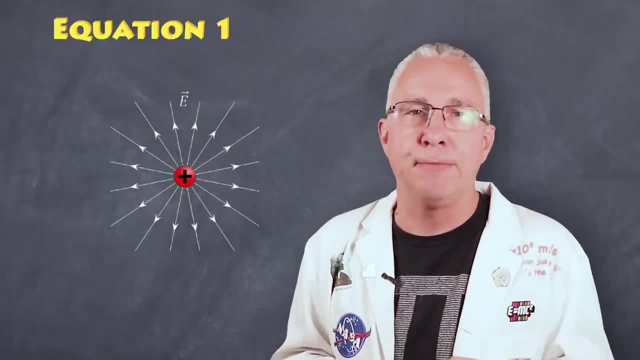 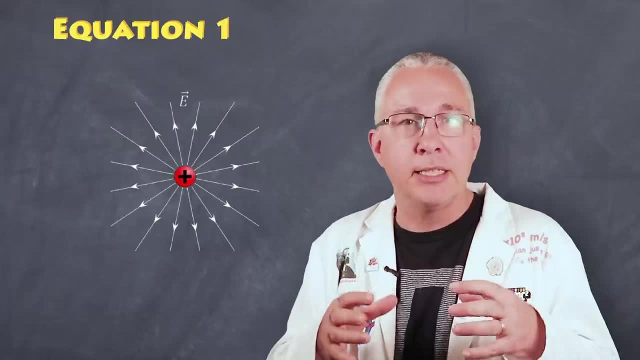 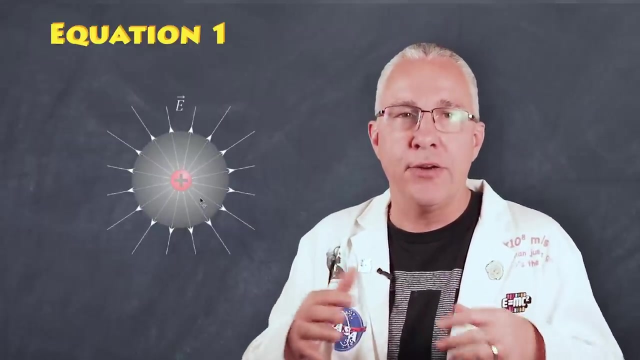 positive point charge has a radiating electric field around it and its value is determined by the distance from that point charge, But the number of field lines, or correctly, the electric flux, doesn't change. That is as you move away, since the field lines are always perpendicular to the surface area of any 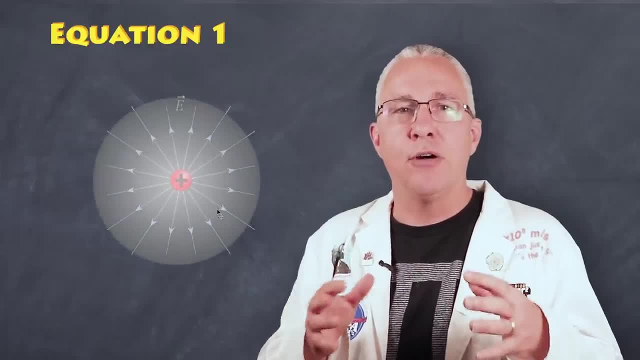 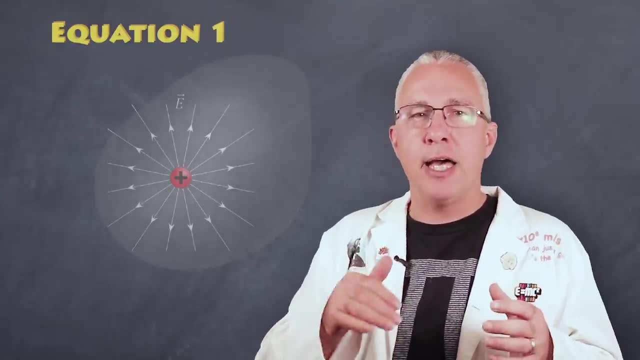 sphere. it's pretty easy to calculate the value of the strength as the flux per unit area, But what if the surface is not a sphere? In essence, if you divide the surface into two parts, the surface is a sphere and the surface is not a sphere. 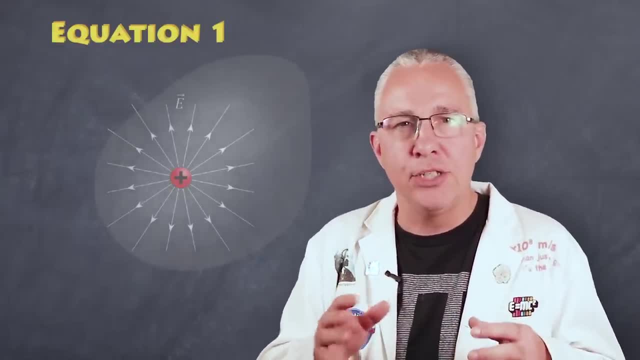 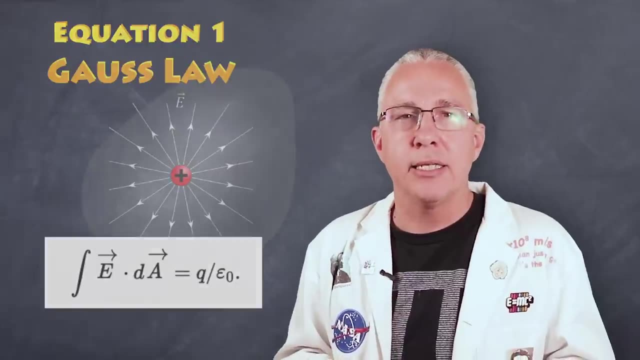 If you divide the surface into two many smaller parts and then calculate the flux lines in each area and then add up these areas, you get the total electric flux for this whole area. In essence, that is what integration does: It divides the surface into an infinite number of smaller areas and then adds them up and 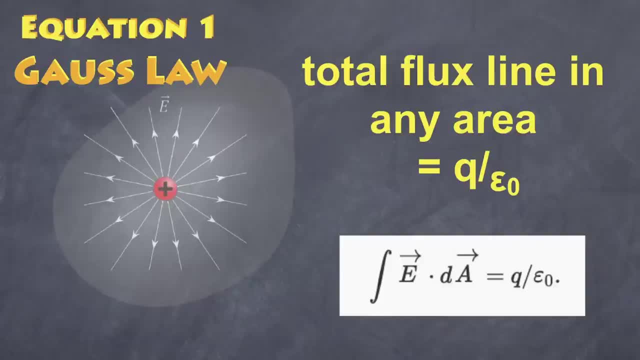 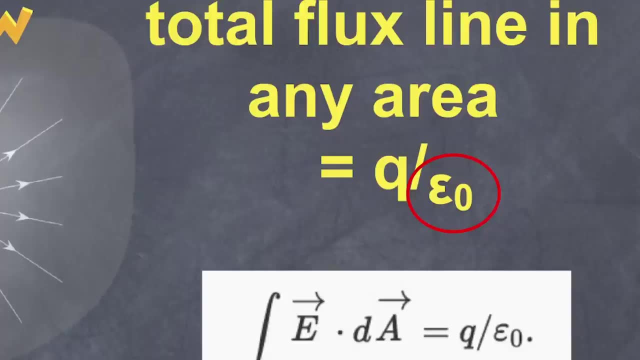 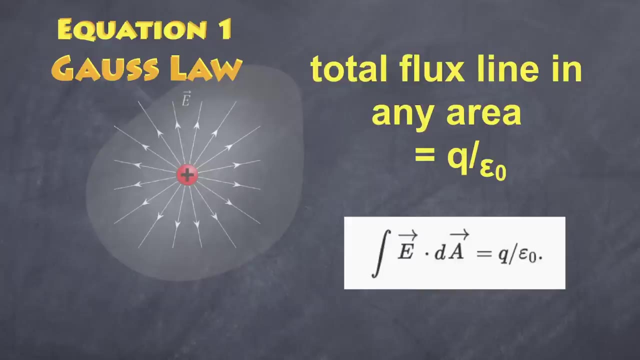 the value ends up being the value of the charge divided by epsilon naught. Now, epsilon naught is the permittivity of free space and it is a universal constant. So no matter what area you have, the total flux is always equal to the charge divided by epsilon naught. The second: 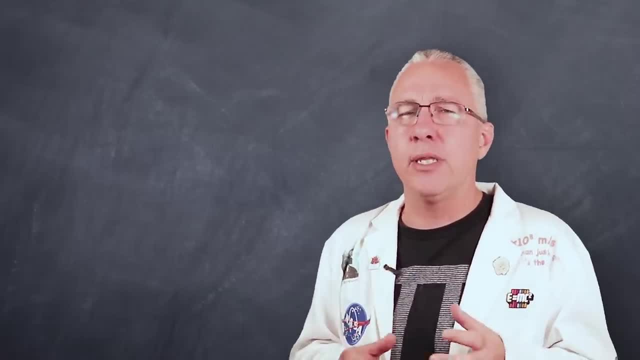 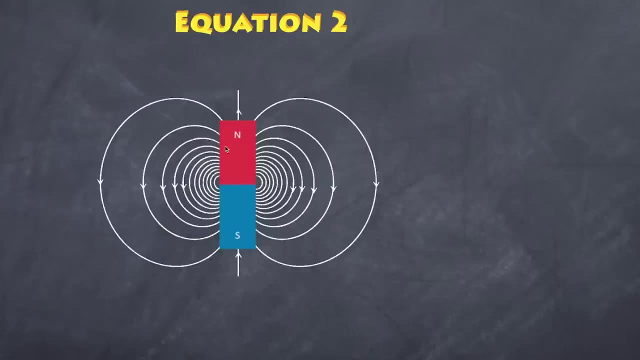 equation is analogous to Gauss's law, but instead of dealing with electric fields, it deals with magnetic fields. So here I have a stock standard diagram of a magnet, and around it you see the magnetic field lines. Now the magnetic field lines seem to start at the north and end at the south, but in actual fact 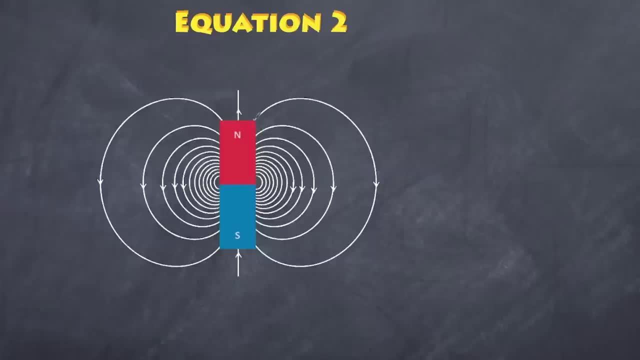 the magnetic field lines are continuous loops, So the magnetic field lines are actually passing through the actual magnet like so. So, in other words, there is no start, there is no finish in terms of the magnetic field lines. They simply go around in a loop. Secondly, the magnet can never be a single pole. what would 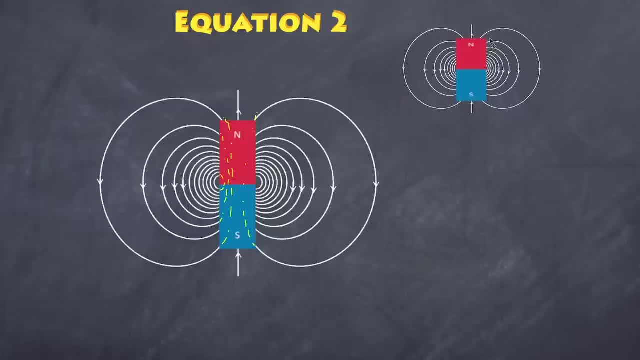 happen if I chopped this magnet in two? Well, I'm going to get two smaller magnets like, so they're going to have a south pole as a result at the bottom and a north pole at the top of the pole pole at the top. In other words, I'm not ever going to get a north pole by itself, a south pole by. 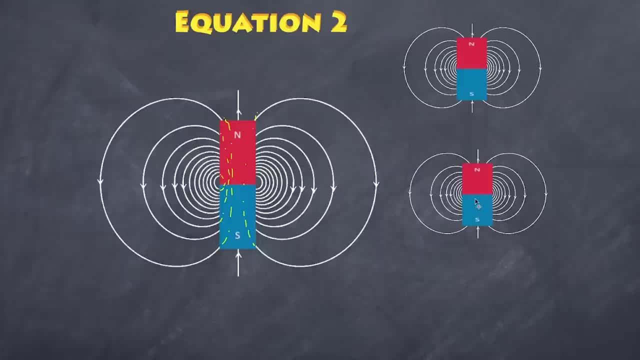 itself, Where there is a charge, where we have a fixed certain charge and lines of force come off it or come towards it. with my magnet it acts like a dipole. You always have two and some lines go from it and other lines go towards it. Which means, if I examine the lines of flux, let's say 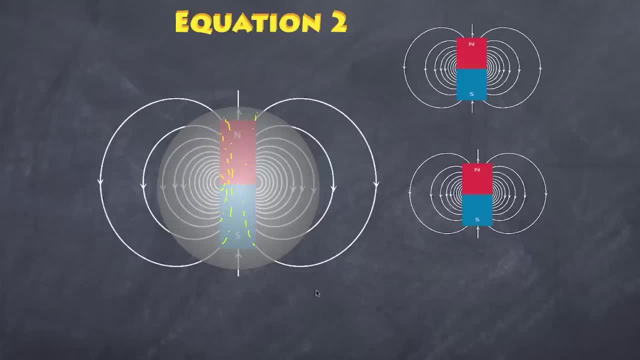 at a particular area and I want to know the total lines of flux on this particular area- and this area can be any shape, for that matter- then I'm going to have some lines of force that are going to be going out and I'm going to have other lines of force that are going to go in, Which means, if 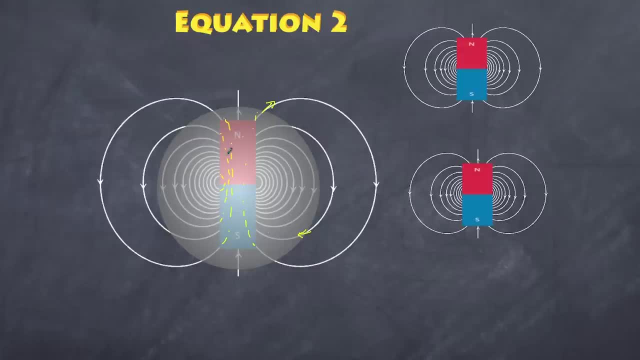 I add up all the lines of force in this situation, because my magnet is a dipole, then I'm going to get a sum total of magnetic field lines, Or flux lines, that are going to add up to zero, And that, in essence, is what the second equation is. 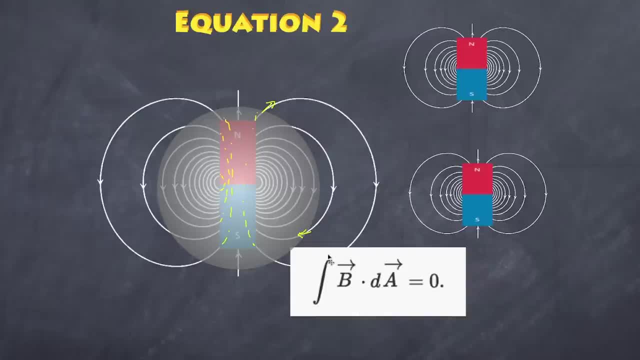 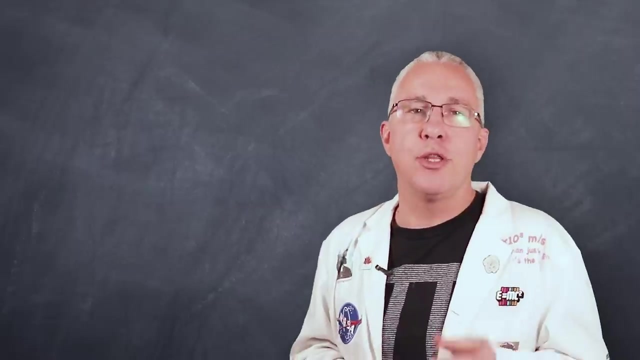 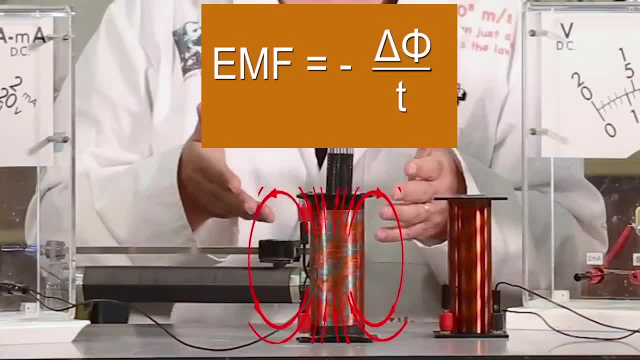 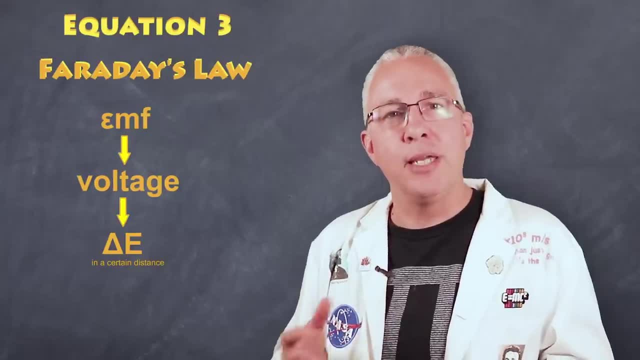 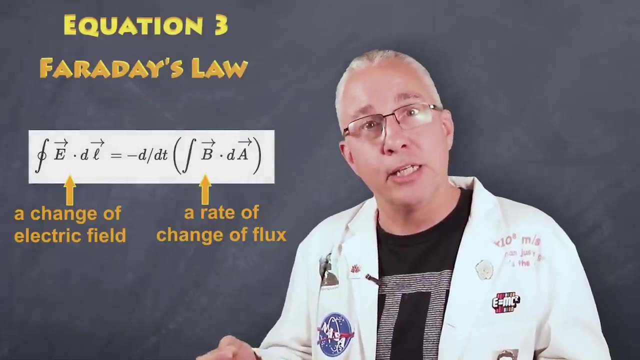 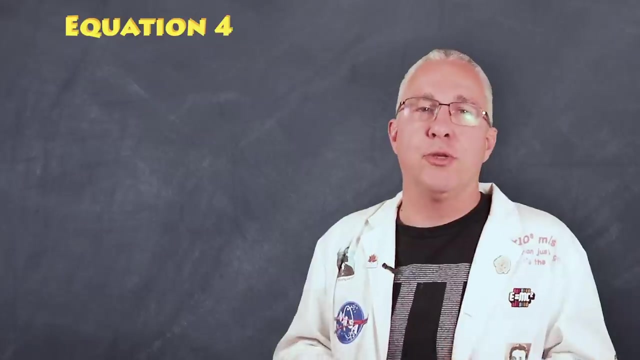 it's a law of induction And it's a law of induction And it's a law of induction And it's a law of. This is called the second equation, which is the third equation, which basically calls the law of induction Right. So start the week and add up that same number of machines and give us 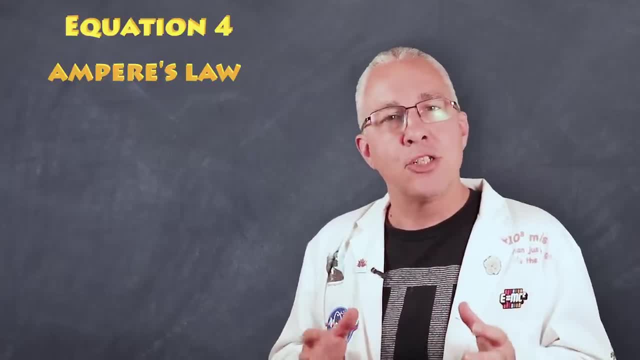 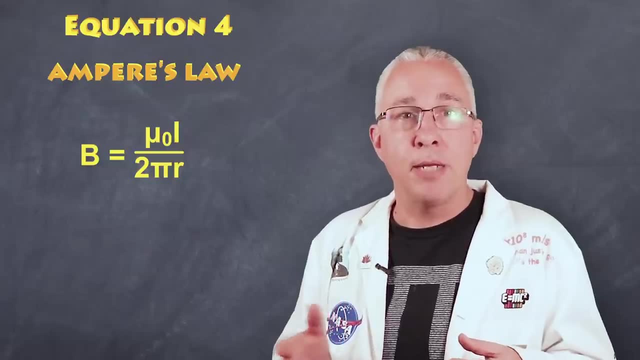 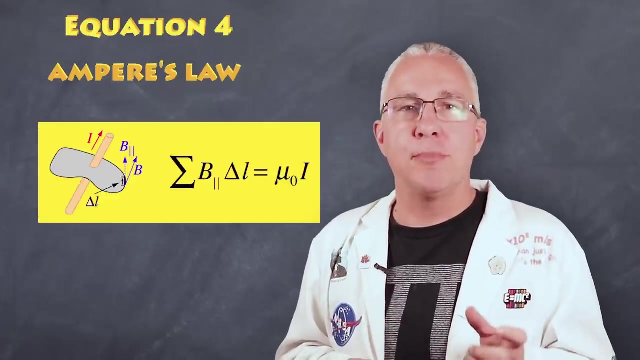 magnetic field around the current bearing wire. Now in the classroom it's often simply taught as the magnetic field strength b equals mu, naught over 2 pi multiplied by the current and divided by the distance. But that assumes that the area around it is circular and Bezlos describes this. 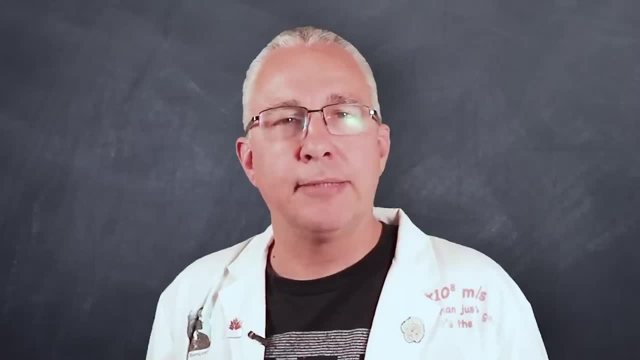 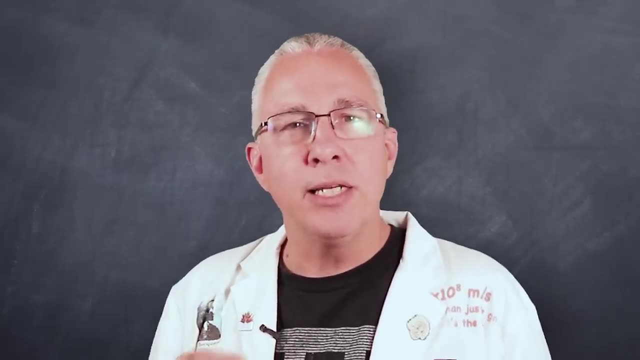 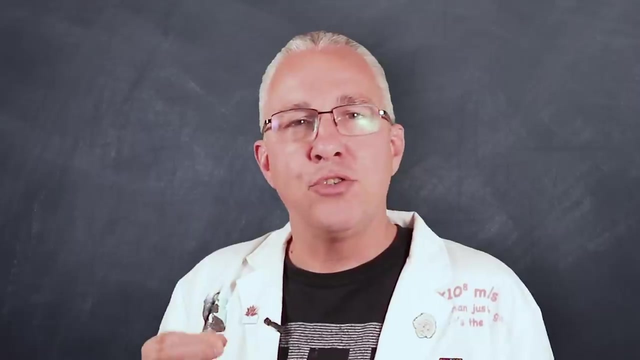 field with any given area. But it's not completely correct because it relies on the current, and thus the field remaining constant. But what if the current changes? When it does, we know that a changing magnetic field will induce an emf and thus a current. So Maxwell's genius was to tweak. 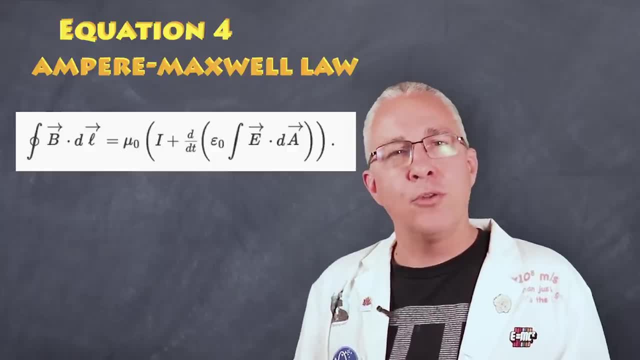 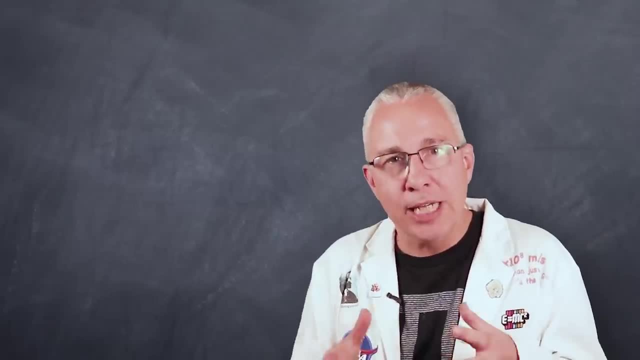 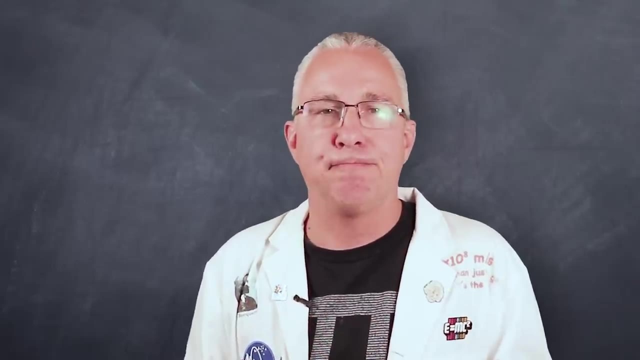 the formula to allow for this. In essence, the fourth equation is Ampere's law, with changing currents and fields considered. So when Maxwell put them all together, he had a mathematical model that intricately links electricity and magnetism. So this is an example of a unifying theory, and 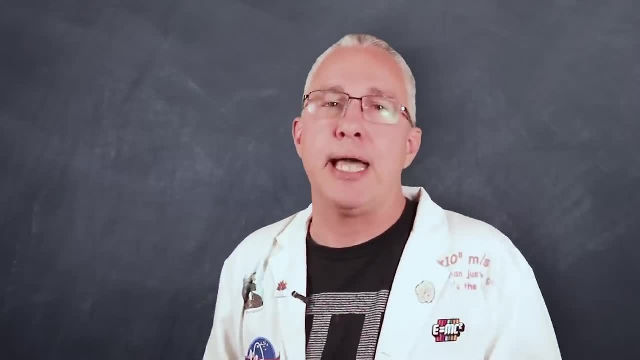 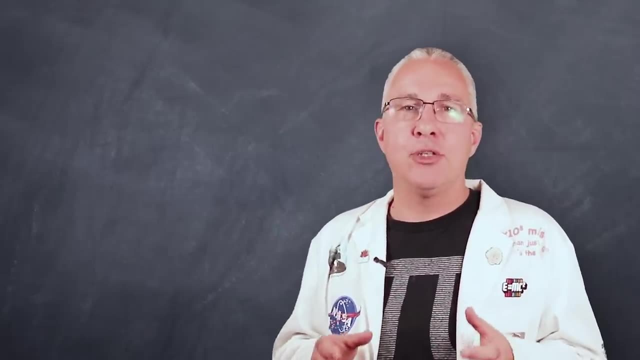 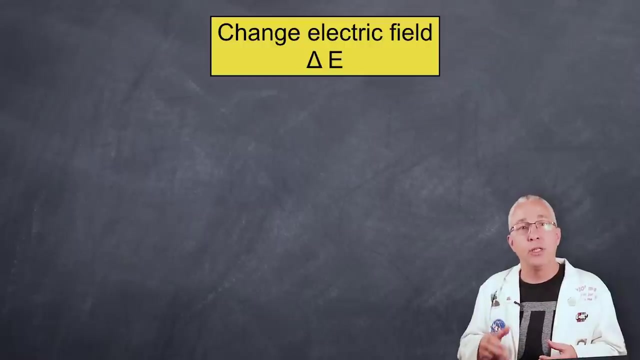 much of physics is a theory. It's about unifying seemingly separate domains. So in this case, Maxwell unifies electricity and magnetism. Now it's at this point that Maxwell took his work a step further to make another discovery. At first he noticed that if you change an electric field, you induce a magnetic field. 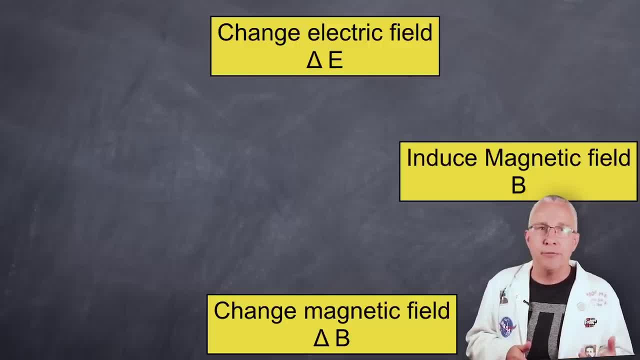 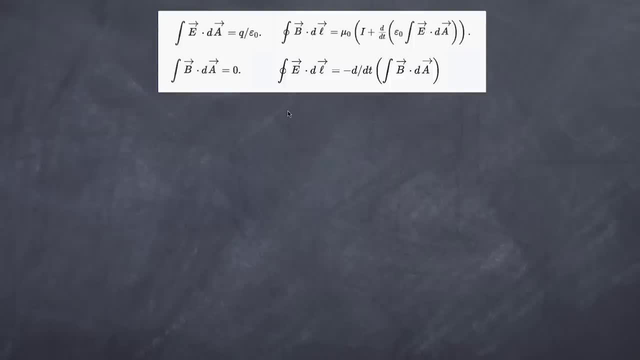 But this changing magnetic field would induce another electric field and this would start the cycle again. What he did next was look at his four equations and he derived the equation, a formula that talks about the electric field and the magnetic field in such a way that they describe. 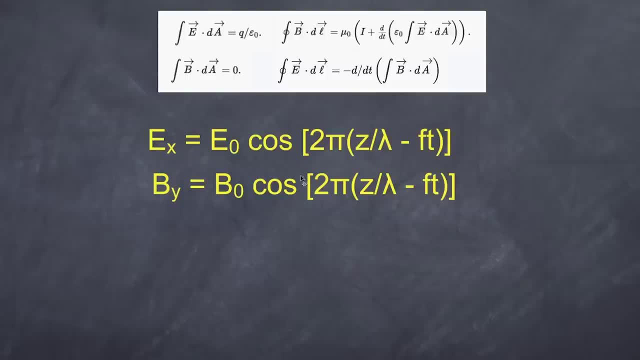 a wave, a periodic wave, And you can see that by this cos term. Now again, I'm going to sound like a broken record here. Do not worry about the mathematics. What's important here is that Maxwell took his equations and was able to describe the relationship between the electric 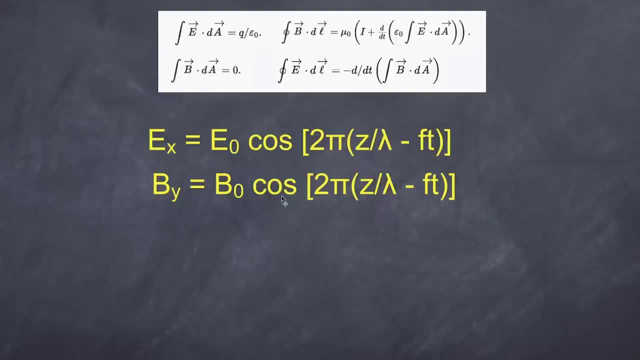 field and the magnetic field in what we refer to as a wave form. In other words, it's generating a wave that has a specific wavelength and a specific speed. And he noted that when the electric field is at a maximum, the magnetic field is at a maximum. 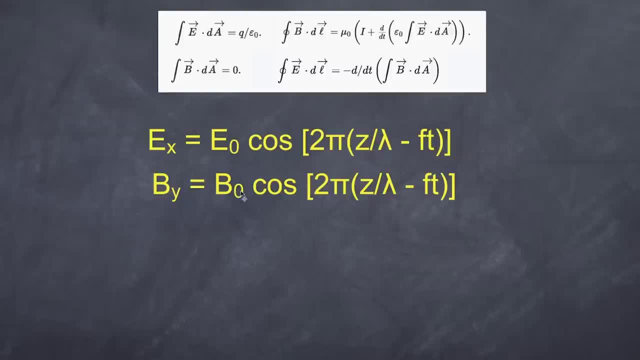 So, in other words, the two waves that are generated, the electric field and the magnetic field, are in phase with each other. Secondly, the electric field and the magnetic field are at 90 degrees to each other And, in fact, because they are at 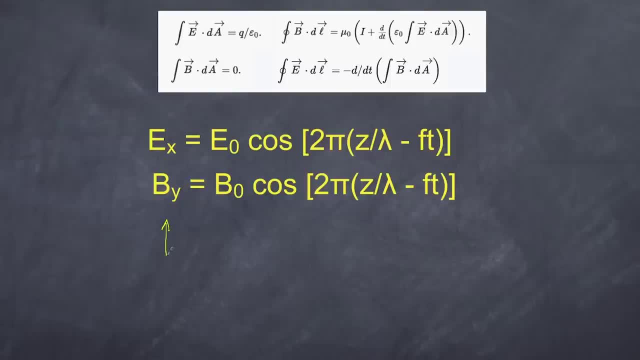 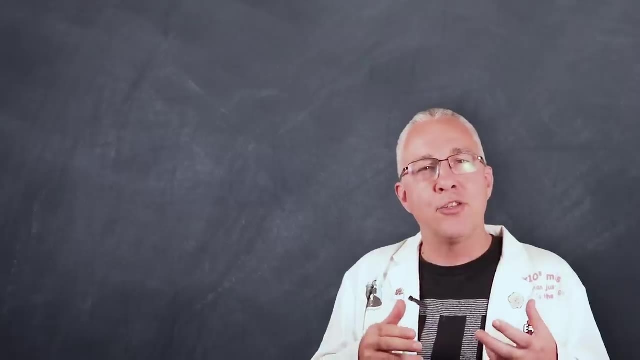 90 degrees to each other. so one is going, let's say, in that direction and the other one is going, is going to go in that direction. That results when those two combined produce a wave that goes in that direction like so. So it has a particular speed. So what you have is a transverse wave that 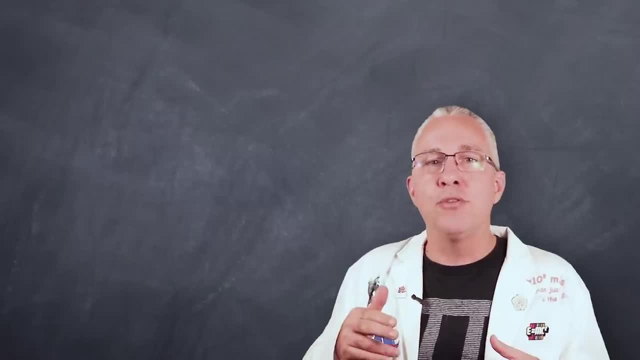 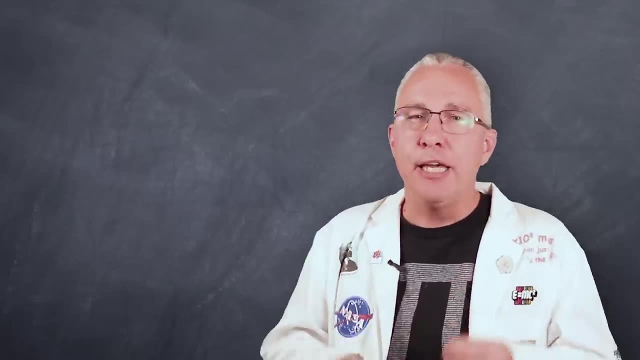 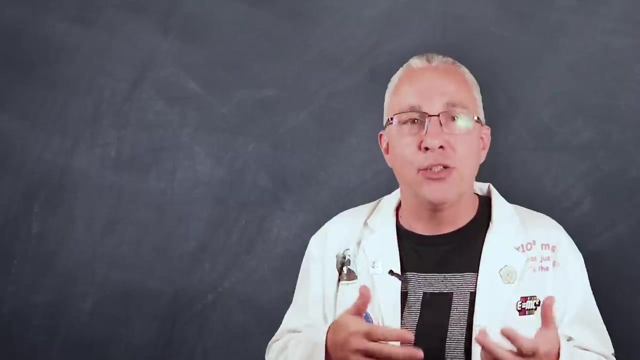 is, in essence, a fluctuating electric field, and this would generate a fluctuating magnetic field at right angles to it, and each field would cause the other. If you start with a charge and you move it up and down, you would generate a wave that would self-propagate, in essence, an electromagnetic 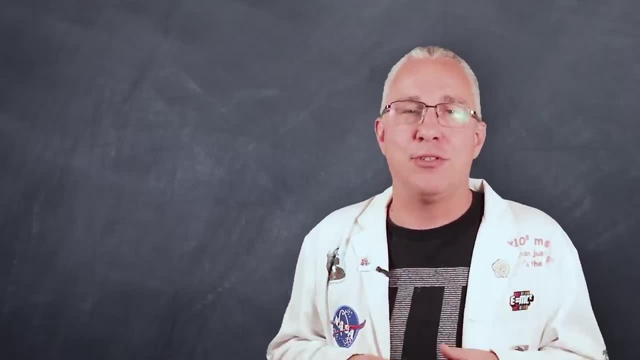 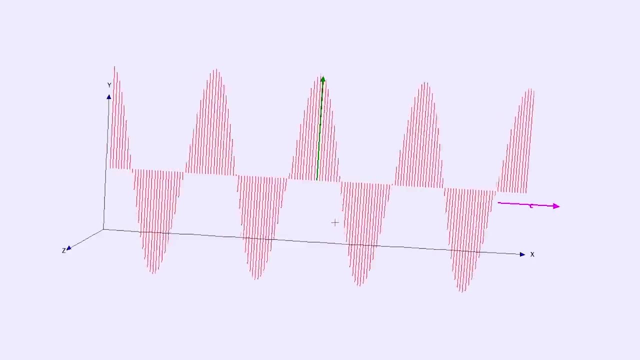 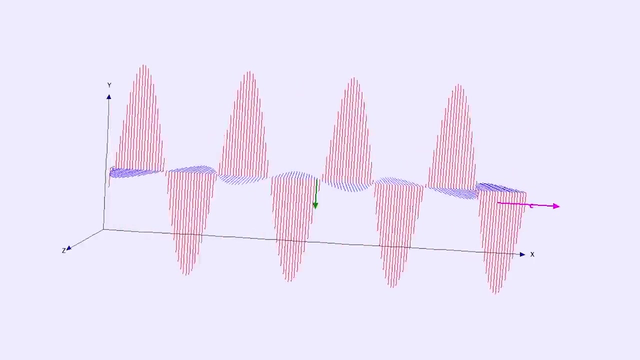 wave. This wave would require no medium, no substance to travel through. So here is our fluctuating EMR wave and we have, here in red, the fluctuating electric field. and, as I said, when we have a fluctuating electric field, we have also a generating fluctuating magnetic field, which 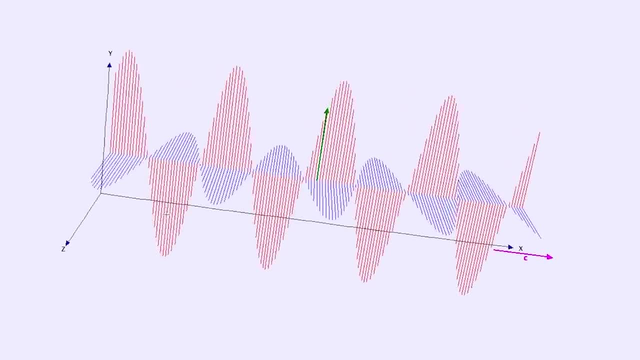 is seen here in the blue. If I change the angle you can see they are 90 degrees to each other and you can also see the just a few more waves that are found as fluctuating material. So a interested, lifezier aurora, So this wave and stagnating. you can see that here in the red parks and sort of. 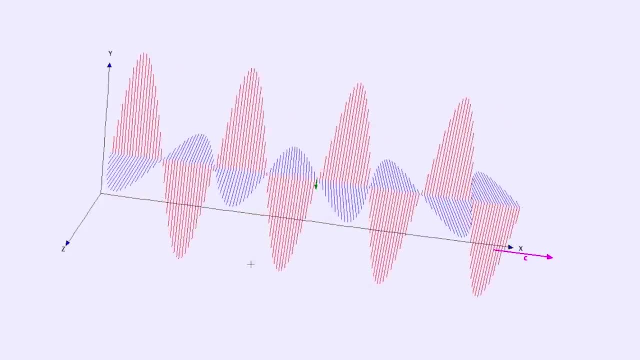 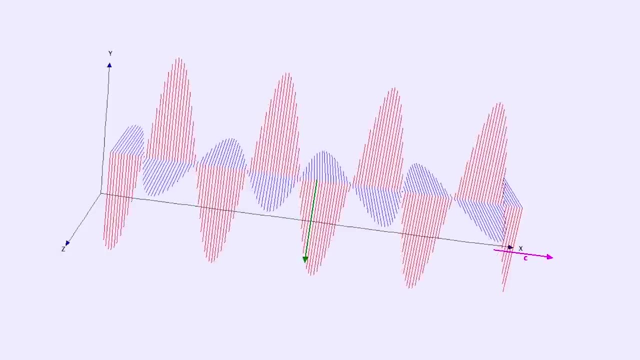 see that when the electric field is a maximum, so is the magnetic field. If I change the wavelength of it, then you'll see that my frequency as a result also changes. So if I have a longer wavelength I have a lower frequency. If I'm going to 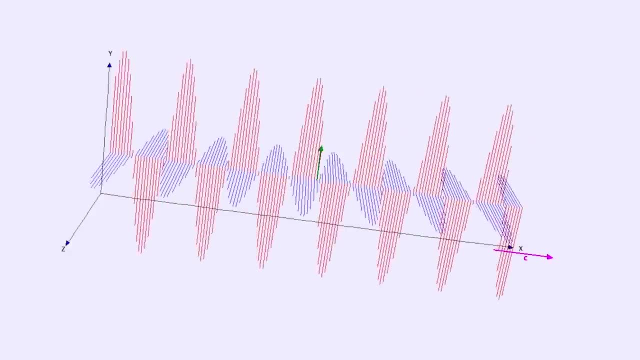 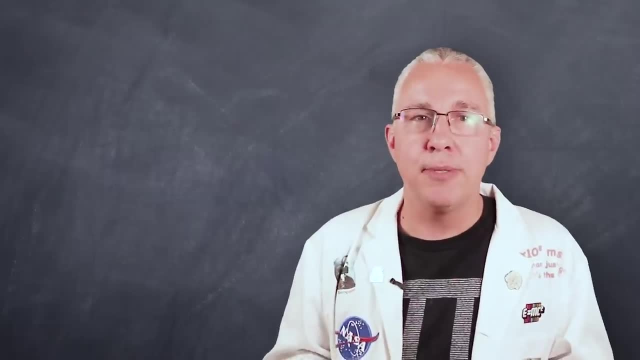 have a shorter wavelength- I'm going to have a higher frequency- and it travels at a set speed. But what is that speed? He then set out to determine the speed of this wave and, by rearranging his equations, he got the speed to be equal.